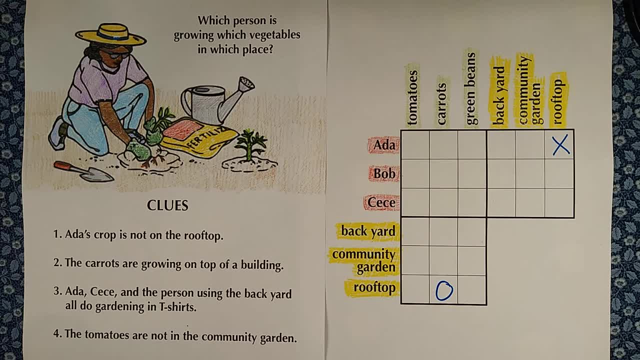 We can write O to mean yes, the carrots are on the rooftop. Then we can put Xs in the rest of the column and row, because we know the carrots aren't in these places and we know these vegetables aren't on the rooftop. Clue three: Ada, Cece and the person using the backyard all do gardening in. 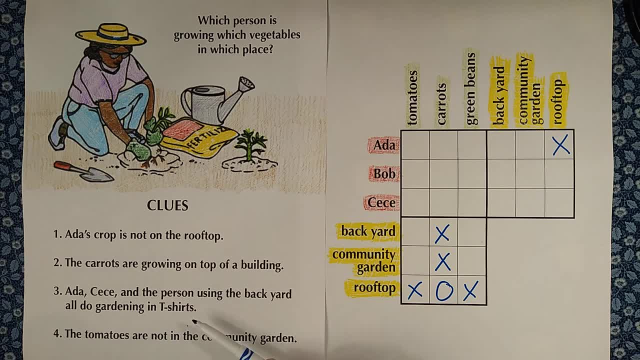 t-shirts. Okay, in every clue, the first thing you always look for is what probably is the most relevant part of the puzzle. The first part is what parts of the clue are in the grid? They do gardening in t-shirts. That's interesting, but what people are wearing is not in the grid. We 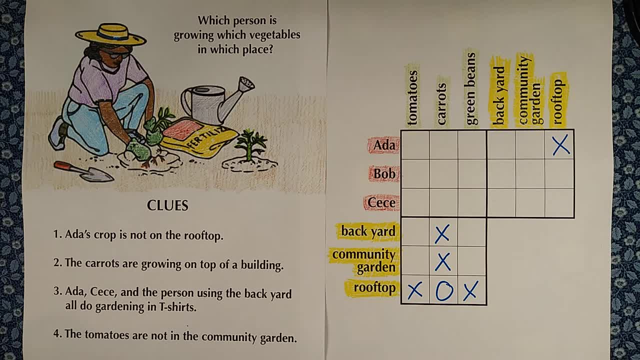 call information like this irrelevant. That means it won't help us solve the puzzle. Let's look at another part- Backyard. That is on the grid. So this information sounds relevant. That means it could help us solve the puzzle. So this is the first clue. The first clue says Ada and Cece. Those names cross backyard here and here. 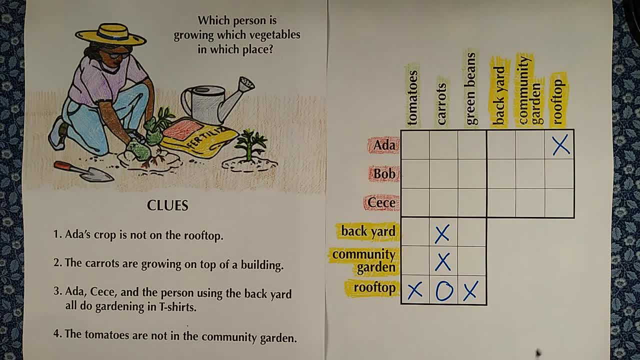 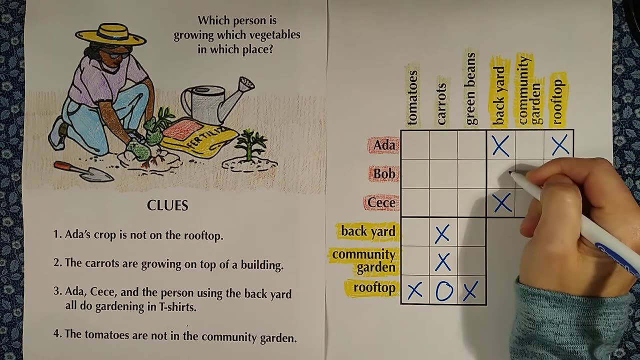 So this clue is pointing to these two squares. What is it telling us? Ada, Cece and the person using the backyard? That means the person in the backyard is not Ada or Cece, So it must be Bob, And that means Bob is not in the community garden or the rooftop. 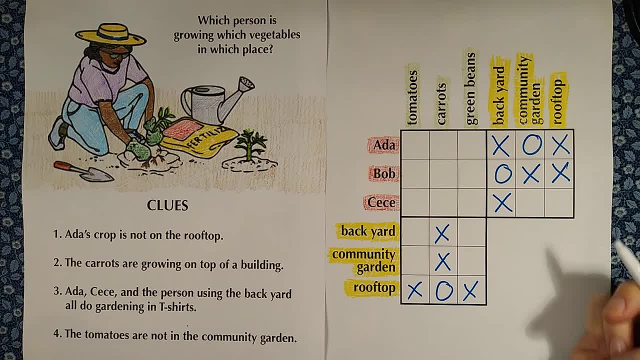 And look at this: Ada must be the one in the community garden and Cece isn't. She must be on the rooftop. Okay, last clue: The tomatoes are not in the community garden. So we can put an x for no in the square for tomatoes and community garden. That tells us. 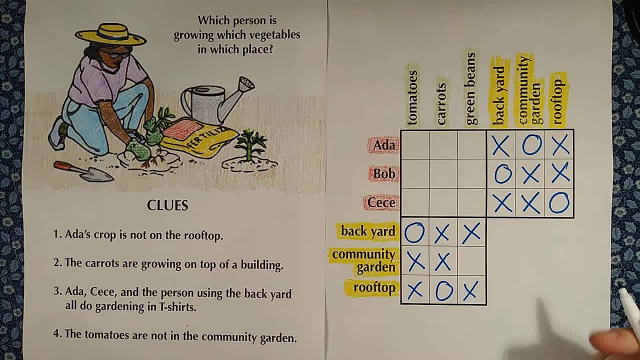 the tomatoes are in the backyard and the community garden. vegetable is green beans. We've finished the clues, but this whole section is still blank. Who's growing what vegetable? To get this, we use these sections to help us. For example, Ada is in the community garden and the squares down here.